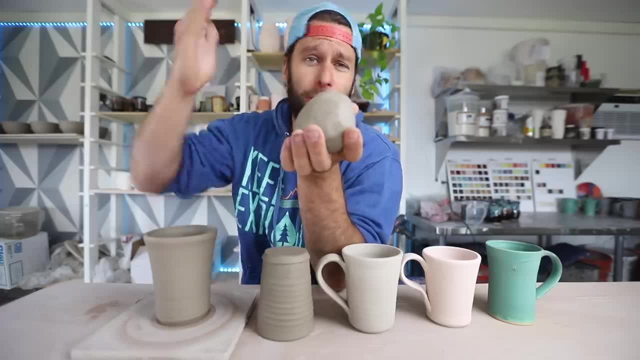 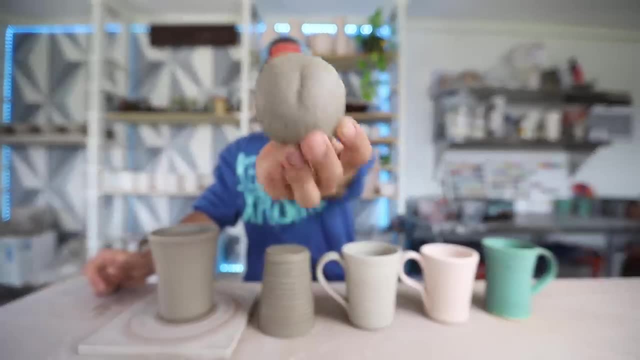 clay from Continental Clay, but there's like a thousand different kinds of clay you can use. You can dig up your own clay and use it, But for the purposes of this video we're starting with this piece of clay. So we start with this clay, We put it on the wheel and 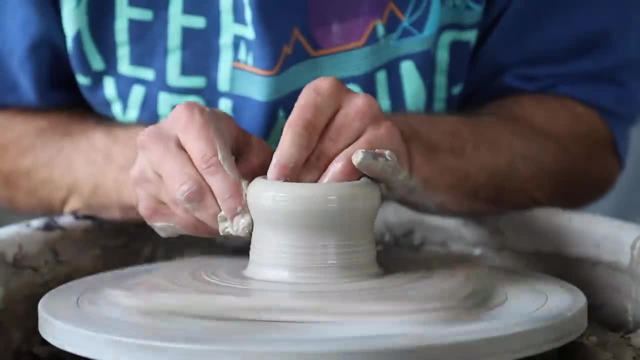 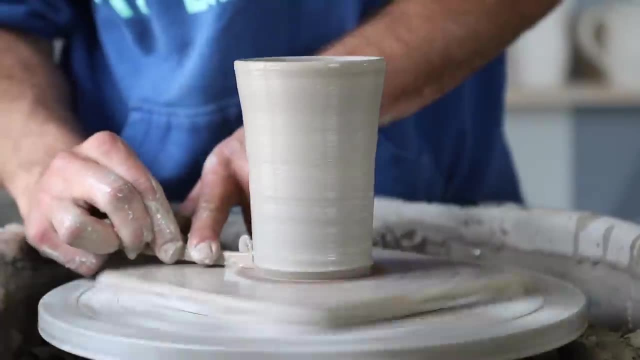 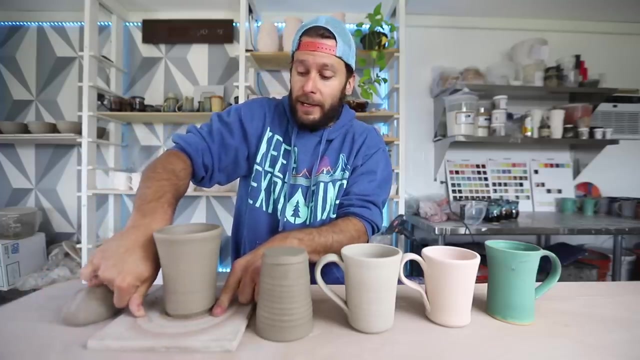 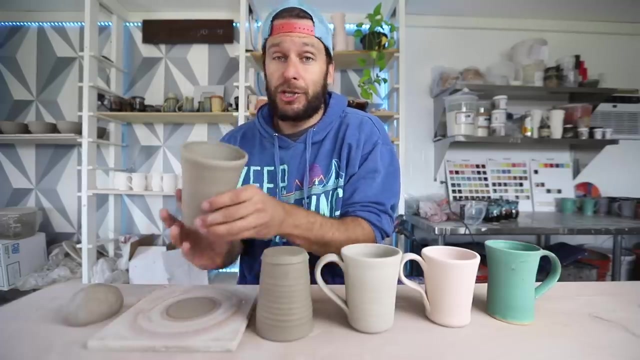 we throw this pot. So this pot I threw like four or five hours ago And one of the most common questions I get is: how do you know when it's ready to flip it over? And my answer to this is: you want to get it flipped over as soon as you possibly can without manipulating. 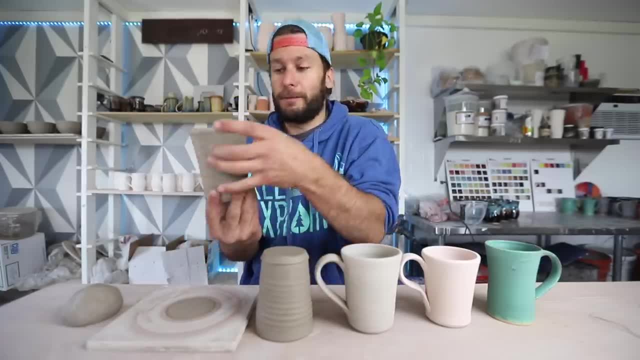 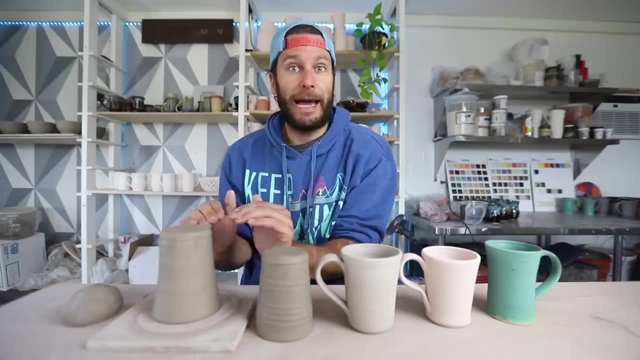 the shape. So like, if you try and move it too early, then you're going to press it and it's going to move weird. So basically you want to flip it over as quick as possible because you want the pot to dry as even as possible. That's one of the biggest things. 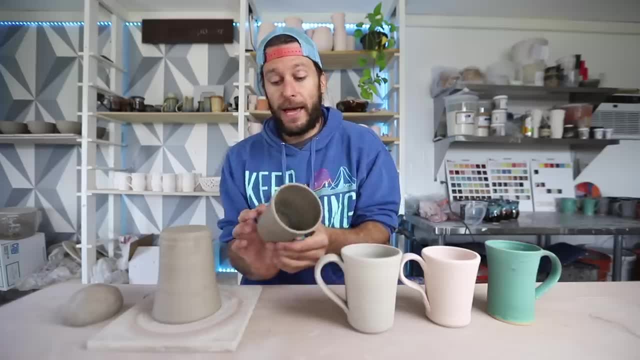 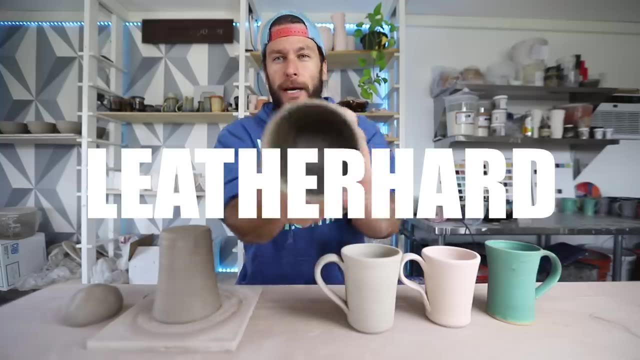 in pottery is you want it to dry as even as possible? Then this pot we threw this morning, this one we threw yesterday, and it's much more firm. It's much firmer than this one. So this one is ready to trim and to put a handle on. 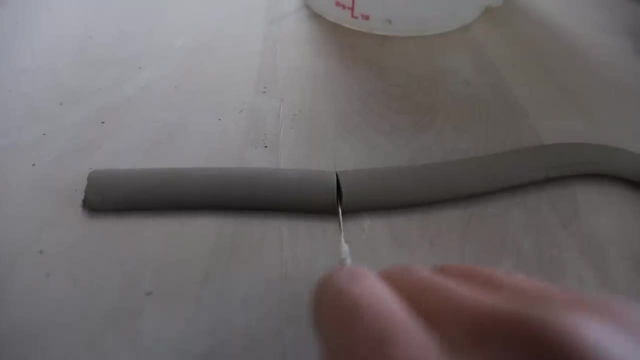 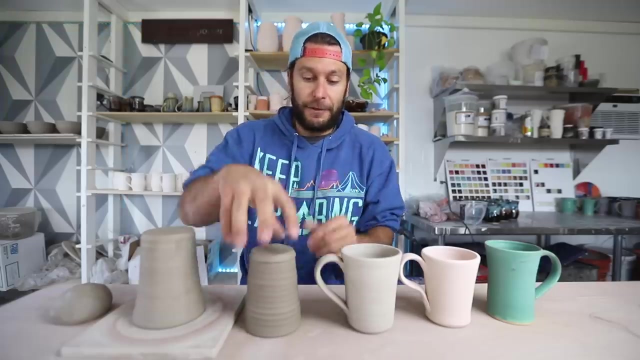 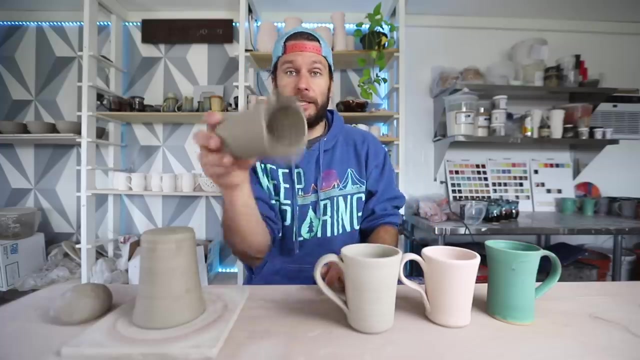 So we're going to do that really quick. The next stage after this, after you put the handle on and you trim it like you saw then, is you let it dry And so this still has moisture in it, but you can't bisque fire it. Bisque is the term. 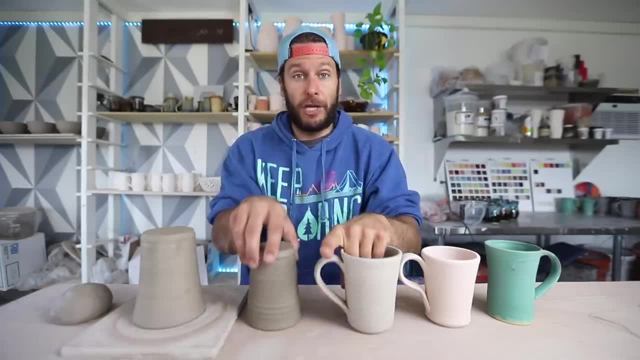 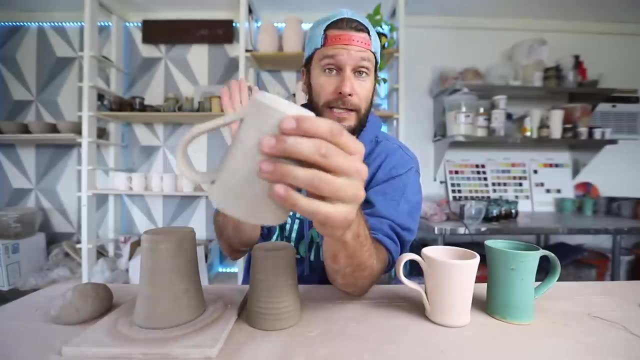 for the first firing, and you can't bisque fire it until it's completely dry, right, Because you don't want any moisture in it. So this is what it looks like when it's completely bone dry. This mug is I made it like four or five days ago It's been sitting and so 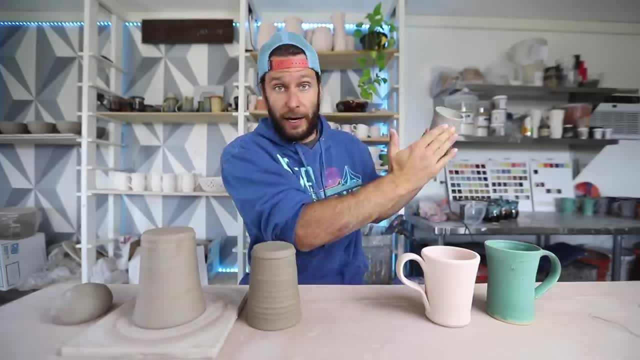 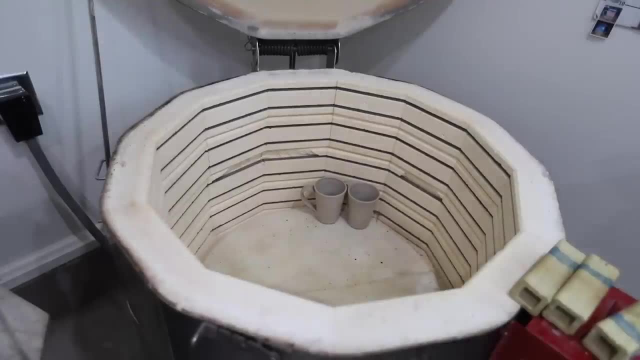 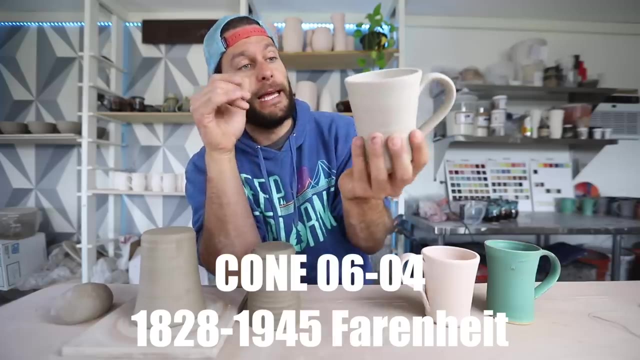 it's completely dry, It's ready to get loaded into the bisque fire. So the bisque fire is the first firing and typically it's at a lower temperature than the glaze firing, So you would. So you put it in there. It cooks for however long. Typically the bisque fire is a slower.